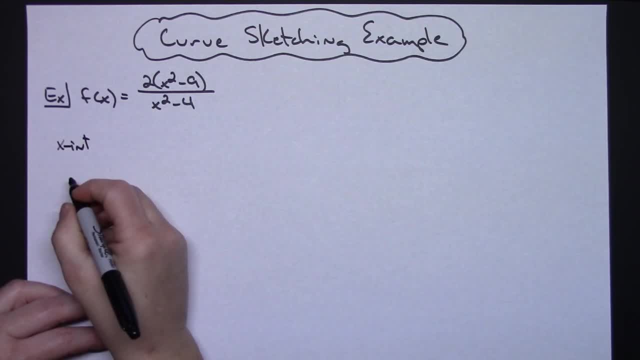 Alright, let's say x and y. we're going to find our x intercepts, all right, which means we're going to set y equal to zero, all right, so we'll go ahead and do that. we're going to have a 2 x squared minus 9 all over that. 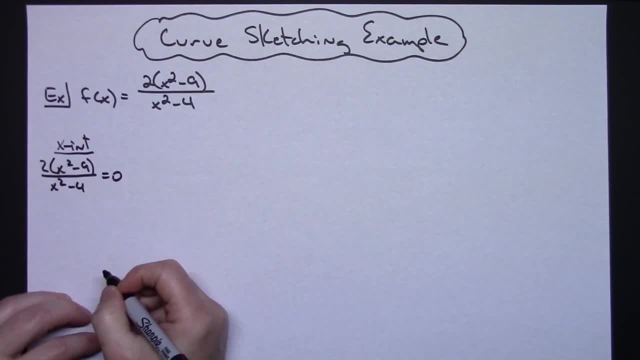 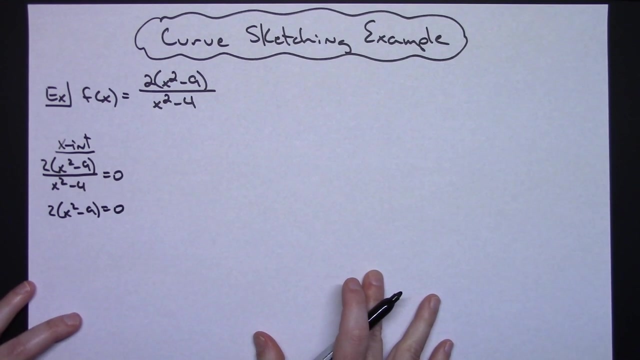 x squared minus 4, and we're going to set that equal to zero, so we can find those x intercepts multiplying both sides by the x squared minus 4. okay, then that'll leave us with the um 2 x squared minus 9 equals 0. i can divide both sides by that 2 and i'll have the x squared minus 9 equals 0. 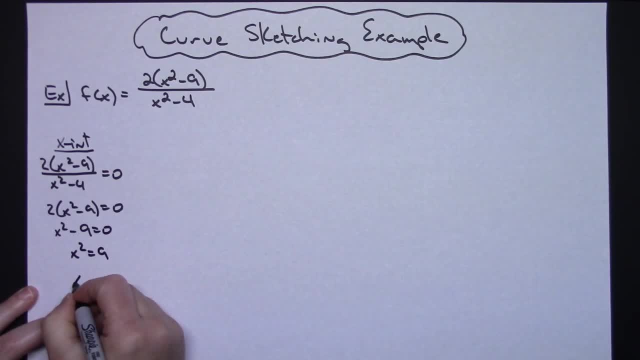 add 9 to both sides and i'm going to get an x equals a plus or minus 3, all right. so then i know i've got plus or minus three, zero for some x intercepts there, okay, and then i have them. then calculate your y intercepts, all right, we know that plugging those. 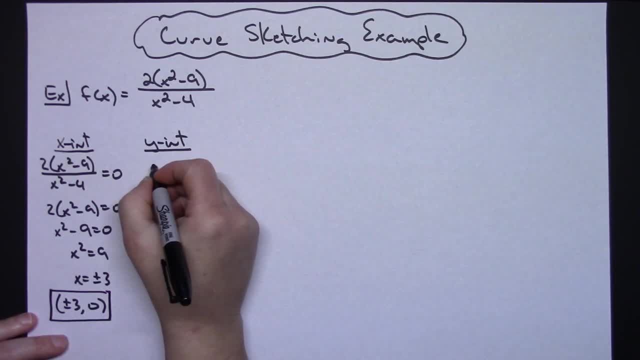 for y-intercepts, plugging in 0 for x. So then I'm going to have a y equals 2, 0 minus 9,, all over a 0 minus 4.. Doing a little bit of math there, we're going to have y equals a negative. 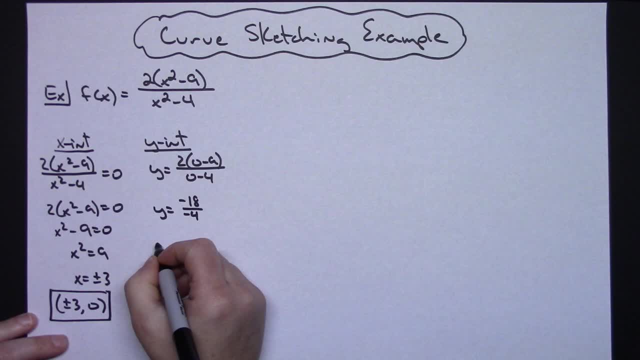 18 on top and a negative 4. So y equals about 4 and a half. So then at 0, 4 and a half we'll have our y-intercept All right. so those are two things that we can really quickly. 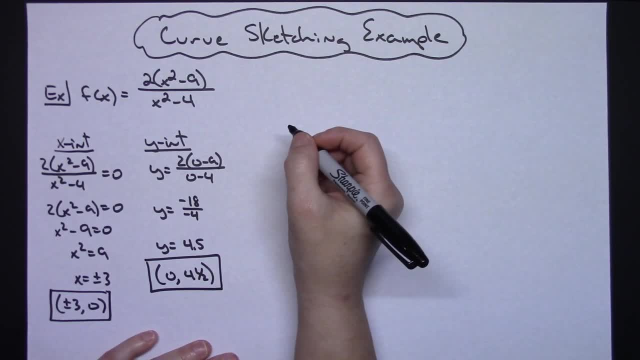 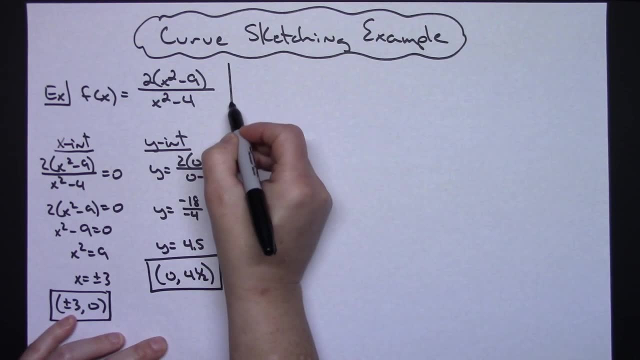 put on our graph. Okay, then I usually have my students look at some horizontal and vertical asymptotes. All right, so here let's box this problem out, so it stays separate from our work. All right, so then looking at our vertical asymptotes, since it is a rational function. 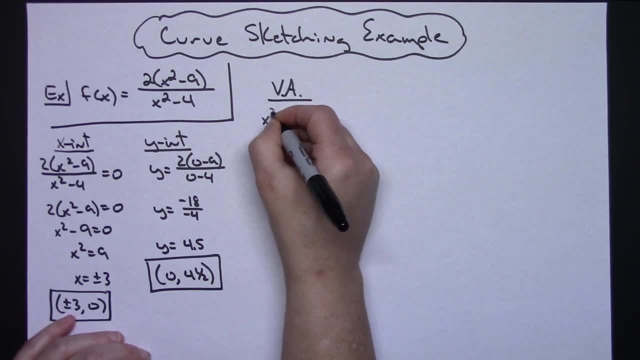 then we know we need to set that denominator equal to 0.. So x squared minus 0, or x squared minus 4.. equals zero. x squared equals four. x equals plus or minus two. So we've got some vertical asymptotes. 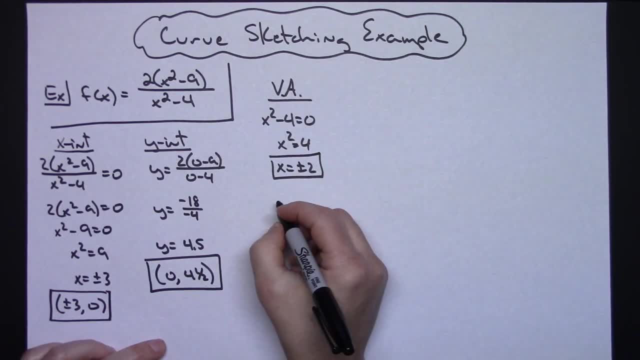 hanging out there at plus or minus two. And then my students know the shortcut rules for finding the horizontal asymptotes of a rational function. If I distribute that on top, then my function is going to look like a y equals a 2x squared minus an 18, all over an x squared minus four. And my 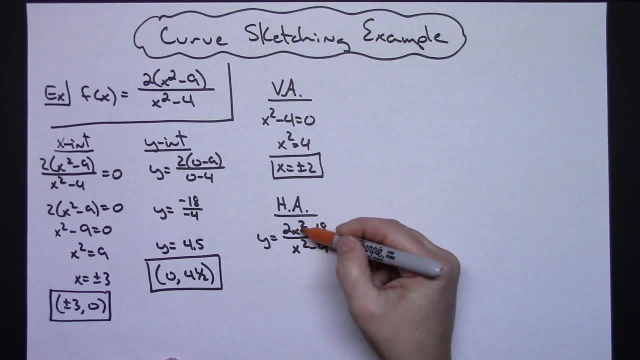 students have memorized that when you can look at the rational function and your power in the top and the power in the bottom is the same- in which case I've got an x squared, x squared here- then my horizontal asymptote comes from those leading coefficients. So I'm going to have a horizontal. 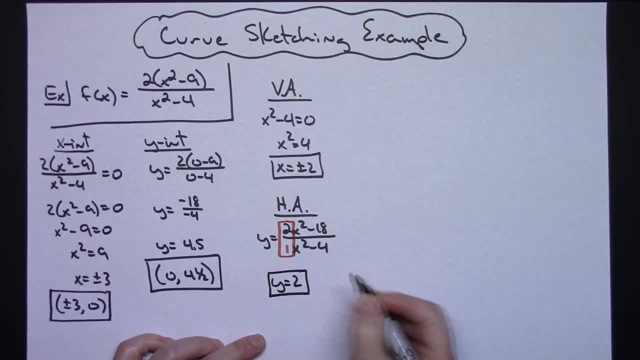 asymptote at y equals two. Okay, so we go through. we probably don't have a lot of time, but we're going to have a horizontal asymptote at y equals two, So we go through. we probably don't have a horizontal asymptote at y equals two, So we go through. we. 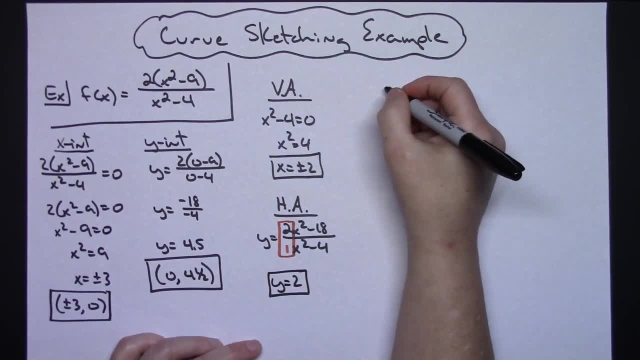 gather a bunch of this type of information. Okay, at this point then, I usually have my students do first derivative. Okay, and I'm not going to take the time to calculate that first derivative, just because that's going to be a quotient rule, It's going to be really, really big, So we'll just 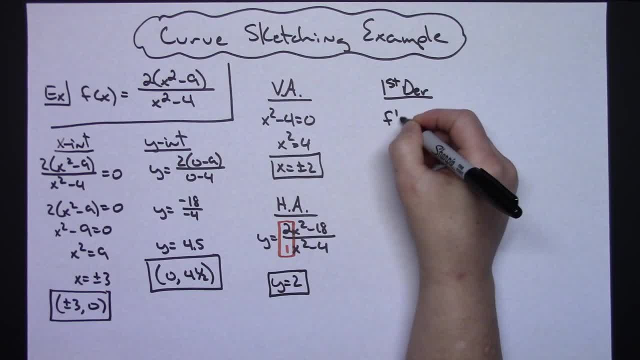 write down here our first derivative. Our first derivative here ends up as a 20x all over an x squared minus four squared. All right, and if you want to calculate that derivative by hand, go calculate that derivative and see if you can come up with that first derivative there After we do. 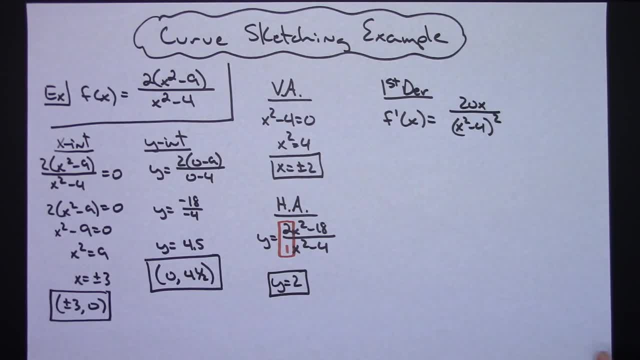 first derivative. then I have them find critical points, because we are going to use a number line at some point here. So it is a rational first derivative here. So we set our numerator equal to zero and we get x equals zero as one of our critical points, And then we set the denominator. 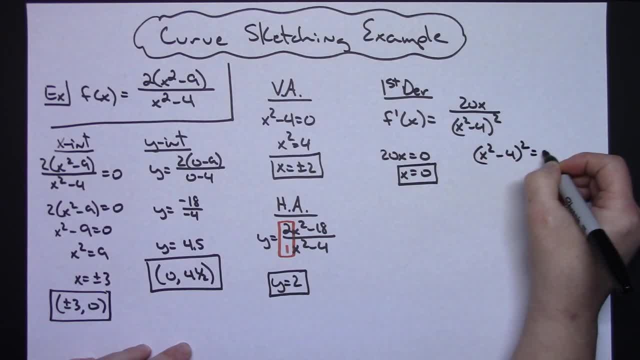 equal to zero. So x squared minus four, quantity squared, equals zero. square both sides, add four to both sides, So x squared equals a four. So I'm going to get an x equals a plus or minus two. All right, so then we've got some critical points. Let's go ahead and label those We've got. 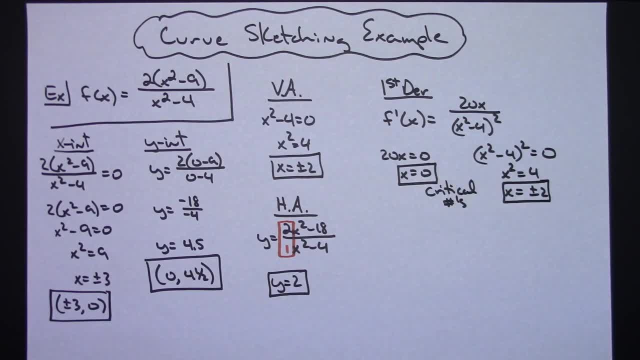 some critical numbers right there, And so on my number line. when I get to that point, we're going to put plus or minus two and zero on that number line. All right, we do actually go ahead then and calculate that second derivative, because we're going to need that in our number line to tell us. 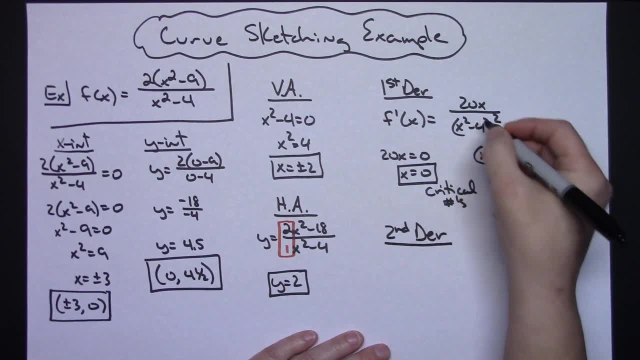 and help with the concavity. And here again it's another quotient there. so it would be quite a long derivative to work out. So I might highly suggest that you pause the video and see if you can get these first and second derivatives. But second derivative here is going to be a negative 60 x squared minus 80.. 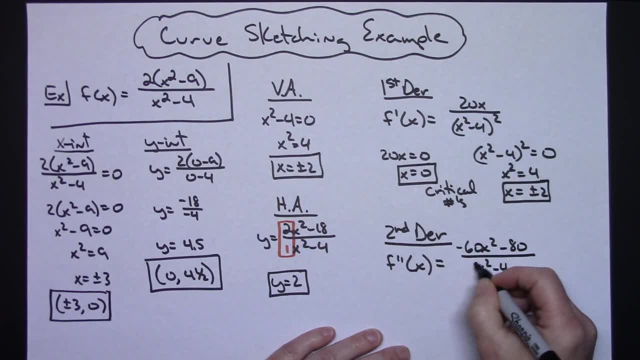 And then we're going to have that x squared minus four to the third power. Okay, and then we would set both of the numerator and denominator here equal to zero. See if we could find some possible points of infinity to be a negative. underneath the square root We can find the negative integral of that square root. 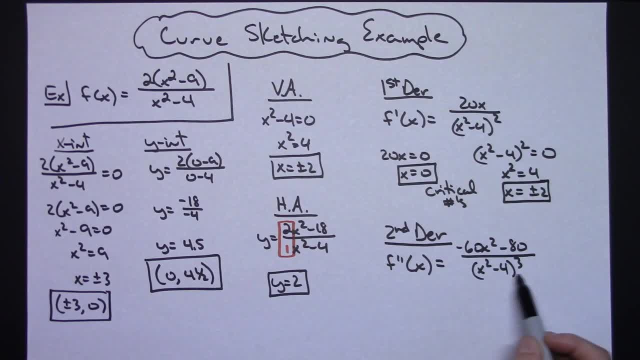 here so we can look at the points of inflection. All right, looking at that numerator right there, it's going to end up being a negative underneath the square root. So there will be no critical points or no sorry points of inflection there from the numerator And this denominator here. 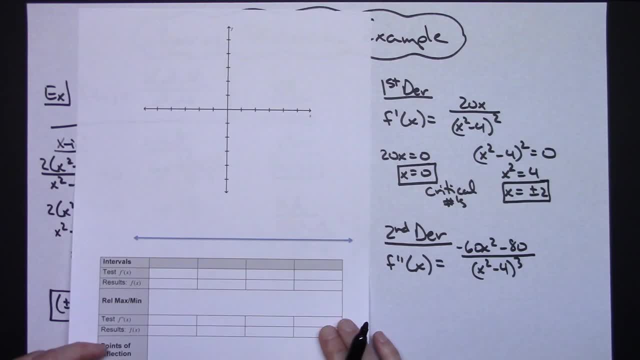 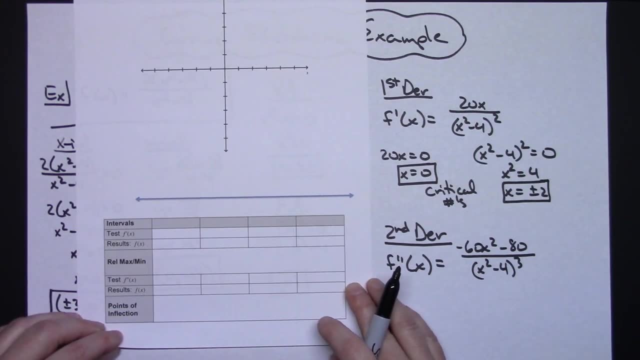 would give me the exact same plus or minus two for points of inflection. So I do not have any additional points that I would need to put on my number line graph paper and then i've got a little chart down here. so usually at this point we have been my. 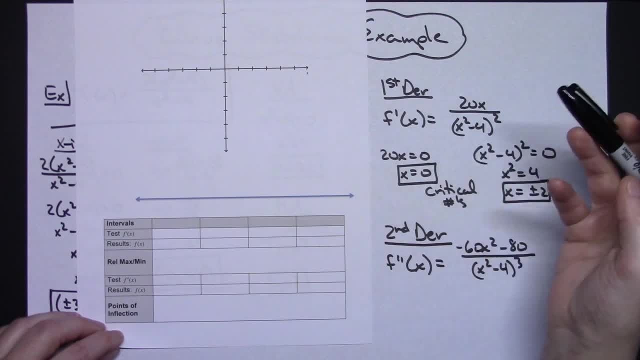 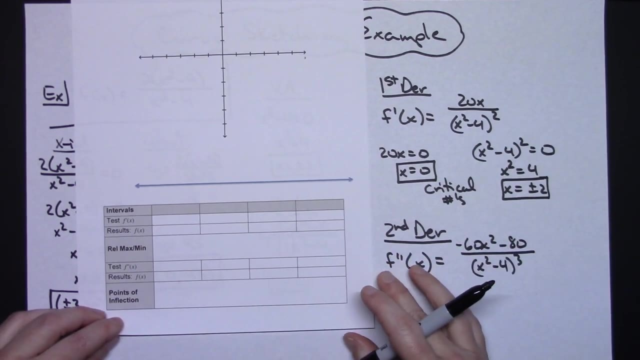 students have been making individual number lines for finding, testing first derivative and finding increasing decreasing intervals. then they have done a different individual number line for finding. excuse me, concavity, you know concave up, concave down. so usually by the time we get to something like curve sketching, then we just make one great big box. here's my number line. i kind of 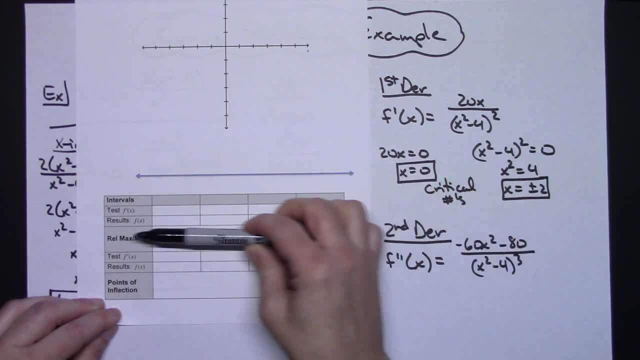 make it kind of organized so that we know that we're we've got intervals across the top. we're testing our first derivatives. that's going to produce some relative maxes and mens. then we take a look at our second derivative and we write our results down. that's going to result here in 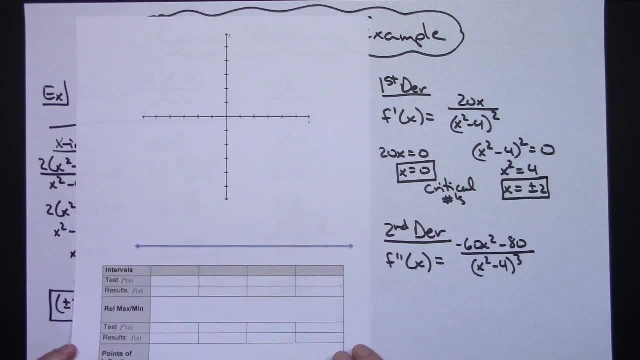 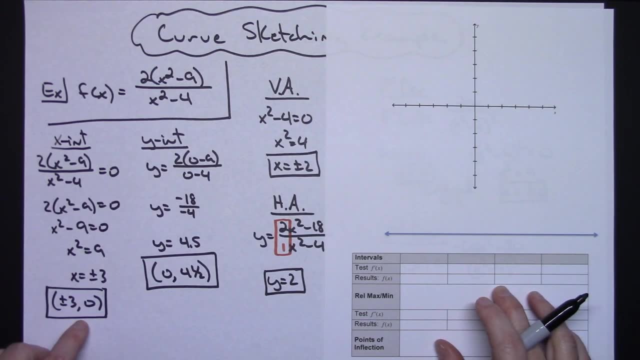 some points of inflection, okay. so, um, before let's come back over here and put on the stuff that we found initially okay, so we said that there were x intercepts at plus or minus three. okay, so i'm going to go ahead and put those on there. so at negative three i've got an x intercept, and at 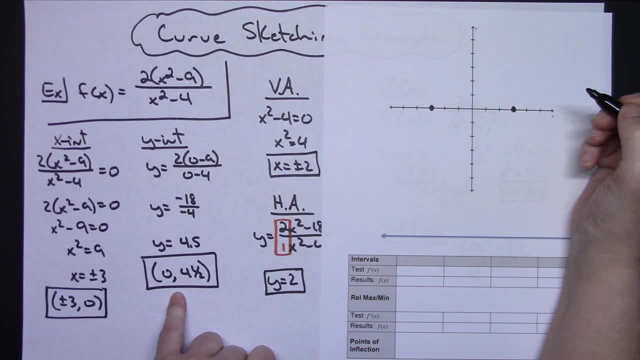 positive 3.. I've got an x-intercept. We also said that we had a y-intercept at 0,, 4.5.. 1,, 2,, 3,, 4.. So roughly right about in there. So get those intercepts put on there. Okay, then the next. 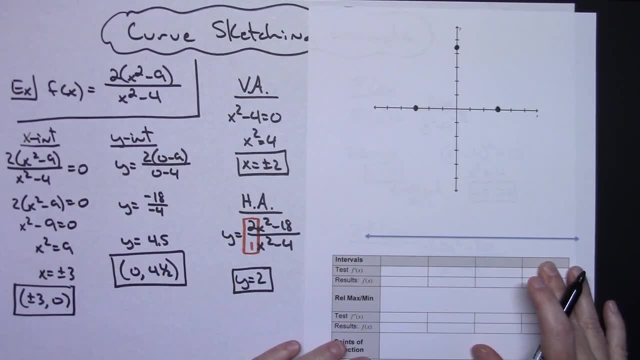 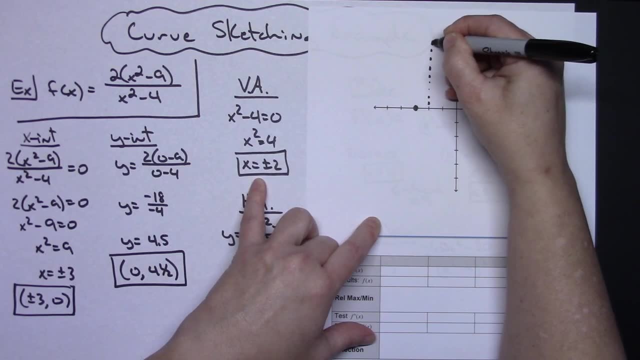 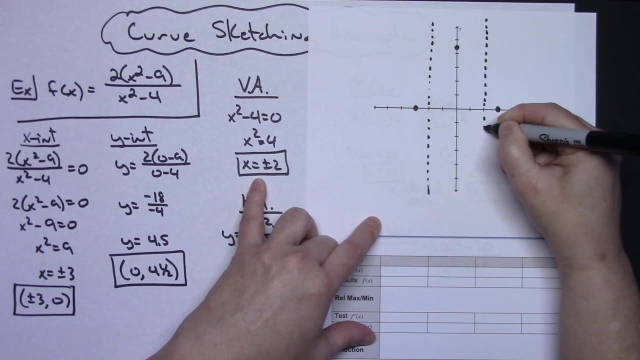 thing that we said we had. we said we had some vertical asymptotes and horizontal asymptotes. So let's go ahead and put those on Vertical asymptotes at negative 2.. And another one at positive 2.. All right, and we said we had a horizontal asymptote at 2.. 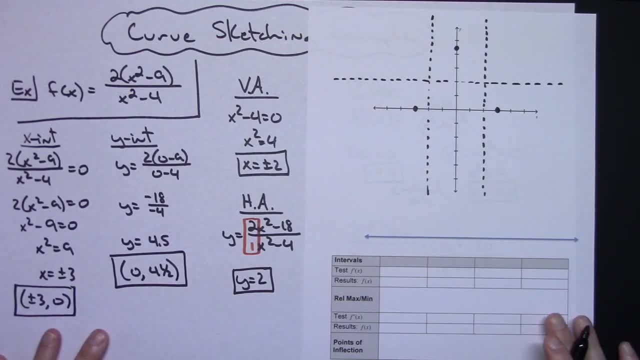 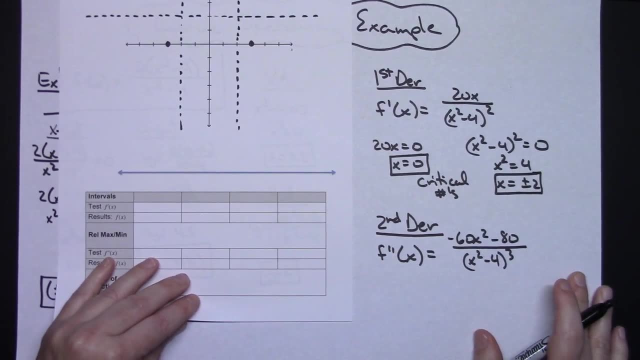 So go ahead and put those things on, because those are really easy, simple things that we can do. Okay, and then now we're going to start working with the calculus part of it. So we're going to take all of these critical numbers and, had there been any points of, 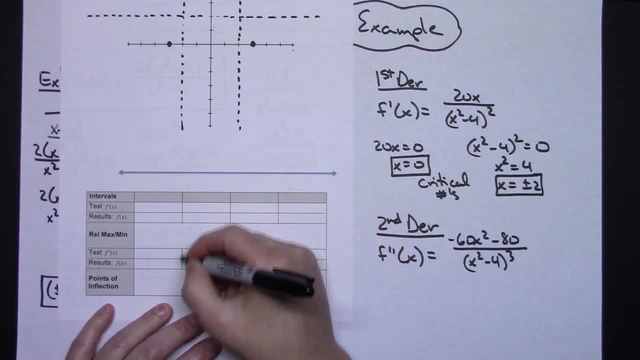 inflection. we would have done those as well. Now, on ours, we line them up here with our intervals here. So I'm going to have a negative 2,, I'm going to have a 0, and I'm going to have a 2. 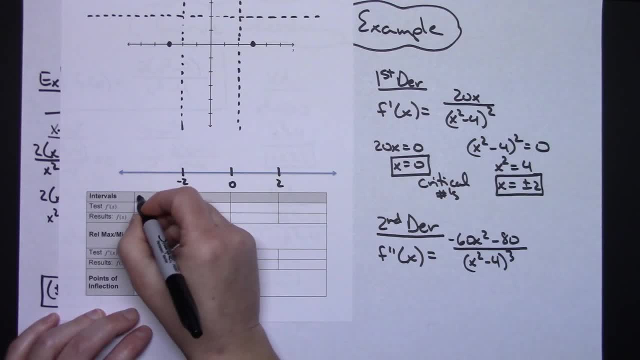 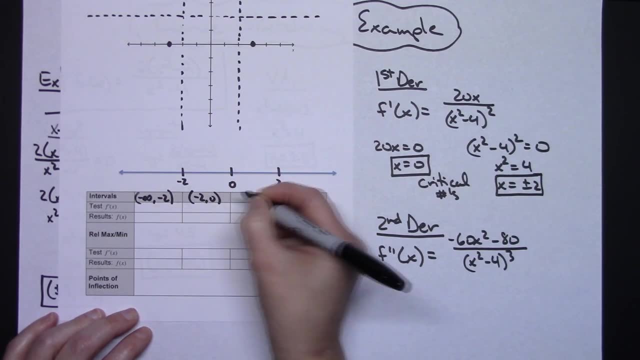 right there. Okay, so that gives me this interval would be negative infinity to negative 2.. This interval would be from negative 2 to 0,, 0 to 2, and then 0 to 2.. So we're going to take all of these critical numbers and had there been any points of, 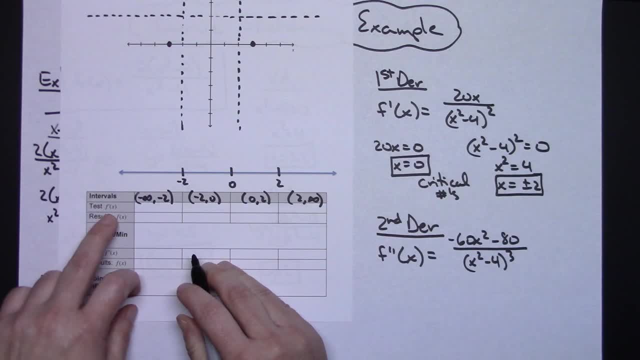 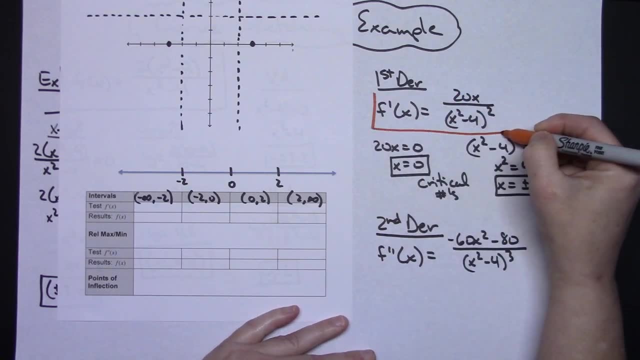 inflection, we would have done those as well. So we're going to take all of these critical numbers 2 to infinity. Okay, all right, now we're going to test this first derivative, All right, so let's go ahead and box that in so it stands out just a little bit there. Okay, so there's the first. 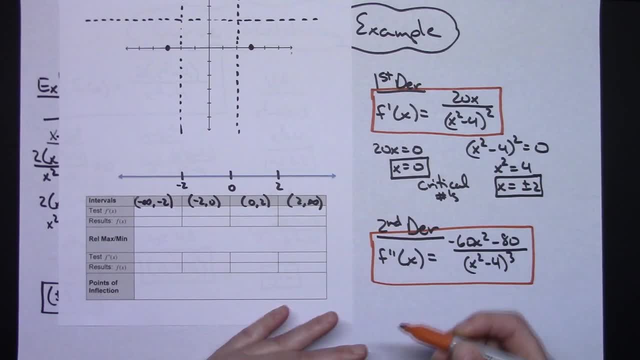 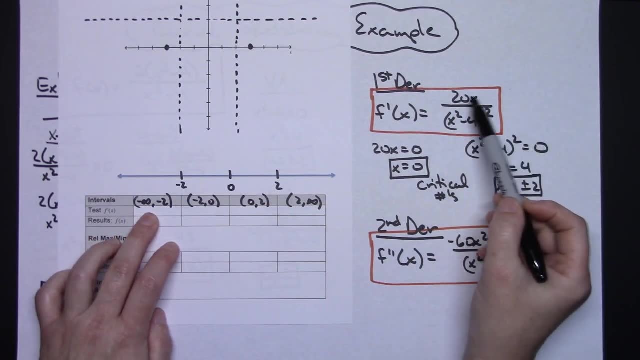 derivative. and here's the second derivative, because that's what we're going to need to be looking at to do these All right. so, first derivative: if I plug a really large negative number in here, I'm going to have a negative divided by a positive. That's going to give me 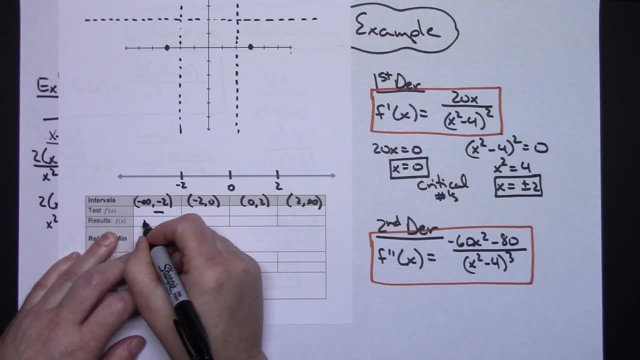 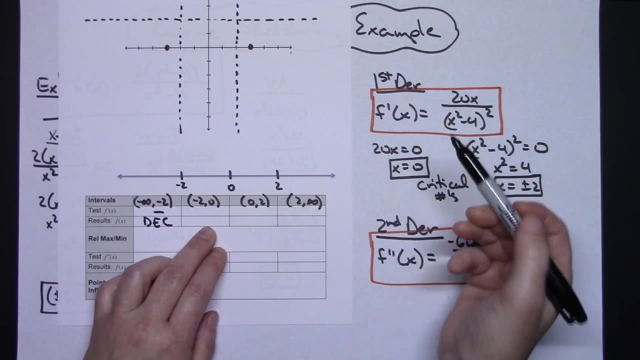 a negative, which means then that original function has to be decreasing In that interval. all right, in between 0 and negative 2, let's plug in negative number again, let's make negative 1.. So again, top is going to be negative, bottom is going to be positive. So 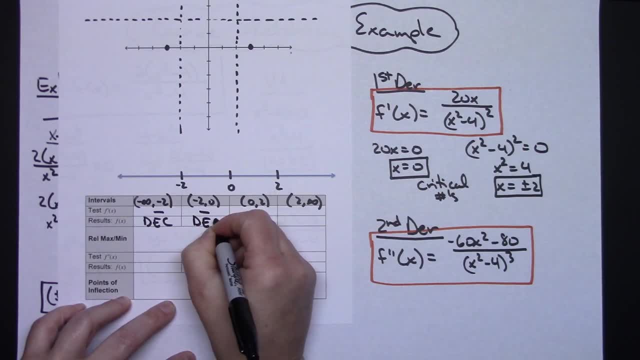 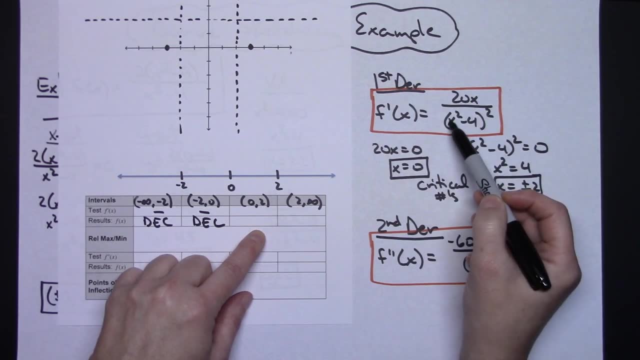 again, this is negative, which makes that original function decreasing. All right, plugging a positive one. that numerator will remain positive and this bottom is going to remain positive too, because it'll be negative, but when I square it gives me a positive there, So I have positive. 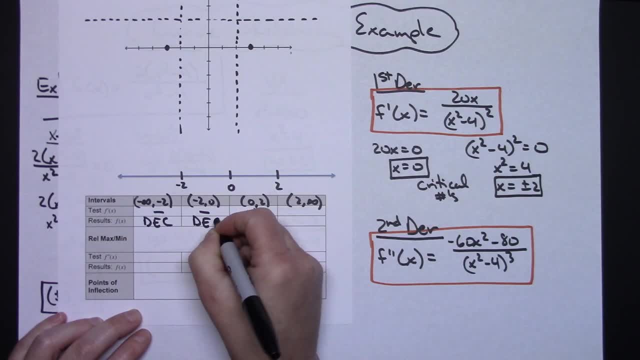 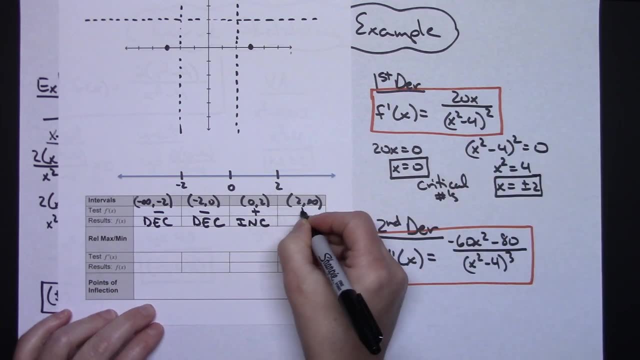 which means my original function is going to be increasing now at this point, and then another big, really big positive number, again positive in the top, positive in the bottom, So positive and increasing across the board. Okay, so then, what that tells me is that when I go from decreasing to increasing, right here at 0,, 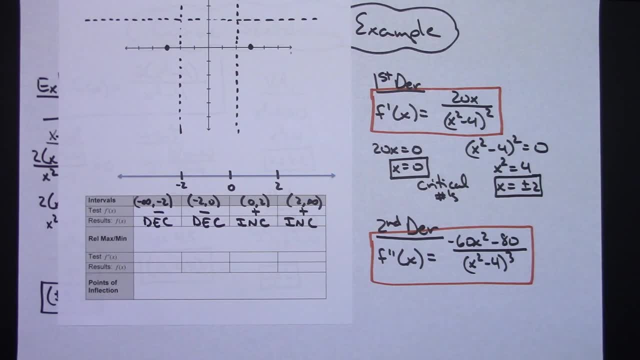 then that has to be a minimum. Okay, so I'm going to put that on there. We need to actually find the ordered pair there. So right here I have a minimum and that ordered pair would be at 0.. Now we're going to have to plug that into. 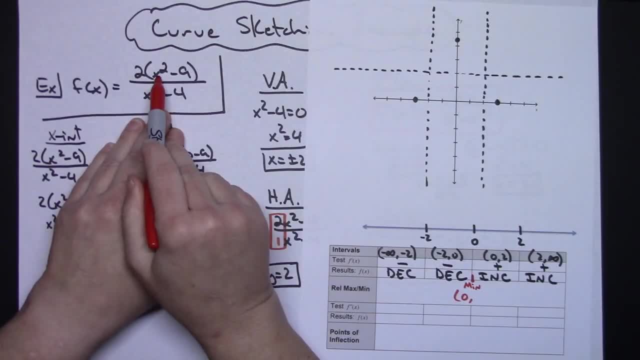 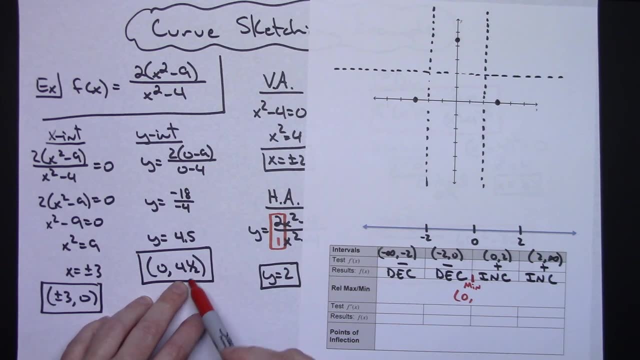 the original function. Let's plug in 0 here. If I plug in 0 here, I'm going to have a negative 18.. Plug in 0 here. I'll have that negative 4.. So that y-intercept that we calculated there. 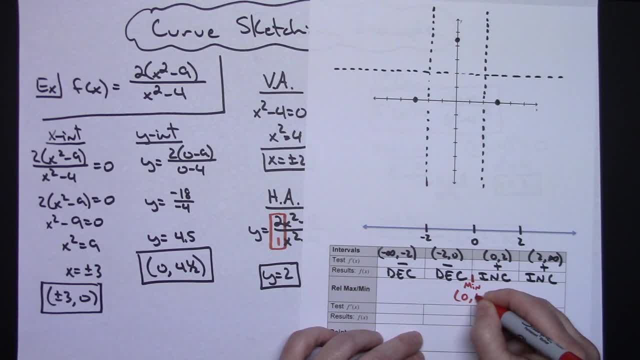 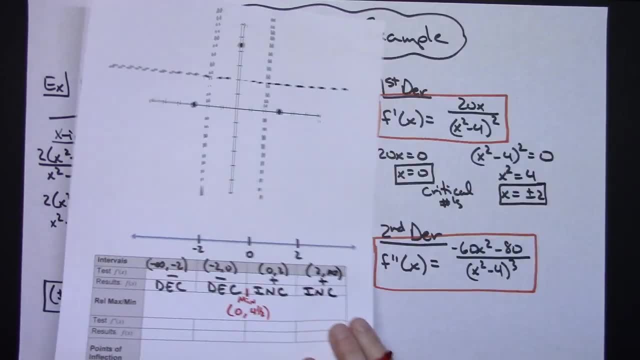 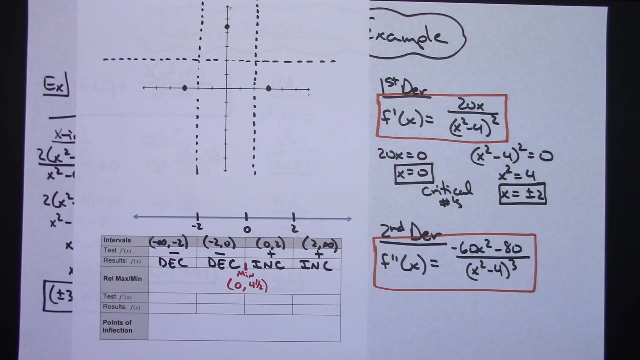 at 4.5 is going to be a minimum. So I've got the ordered pair on the graph. That's going to be a minimum right there. Okay, now let's keep going Right here. we've done the rest of this chart here, All right. now I'm going to have to take a look at the second derivative. 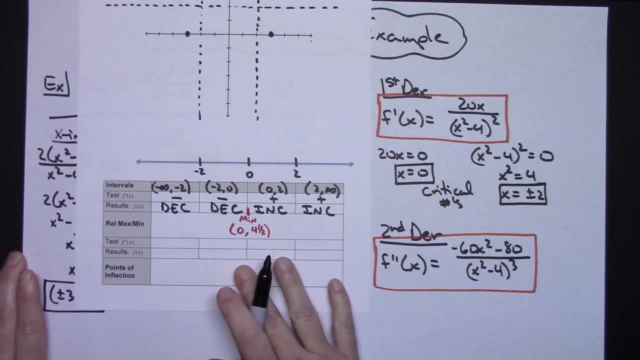 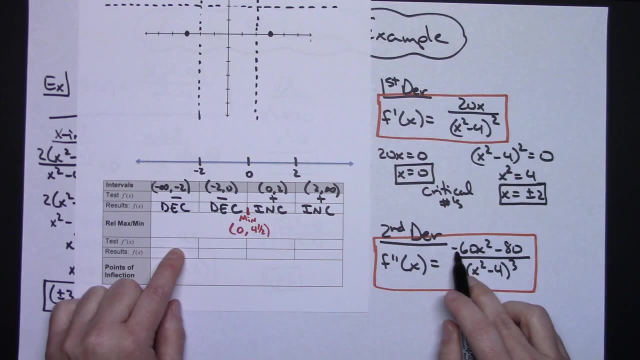 All right. So taking a look at the second derivative, Let's move this up just a little bit there. All right, First derivative: here, If I plug in a really big negative number, that'll be positive. So this is going to remain negative. All right, minus negative. 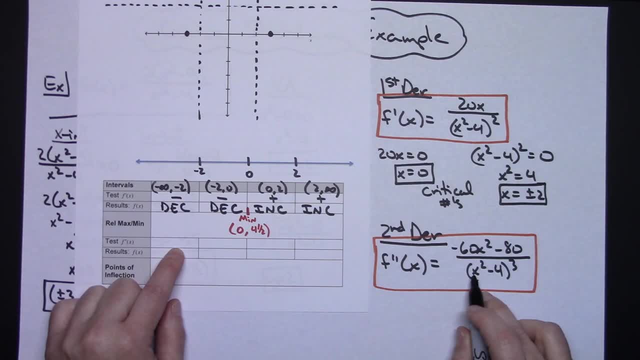 So I'm going to have negative on the top Plug in. It really doesn't matter here, because I squared it. it's going to be positive, but it's going to be really big, so I'll have a positive on the bottom, All right. so negative over positive. 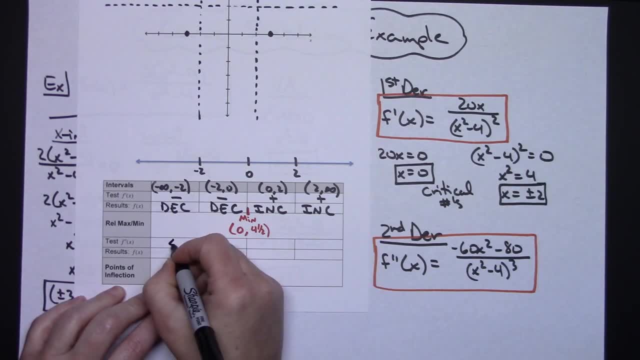 Positive will be unusually in kind cavity. I say less than 0 and when the second derivative is less than 0, then I have a Concave down on my original function. all right, plugging in a negative 1 here again same, It's gonna be the wait a minute. 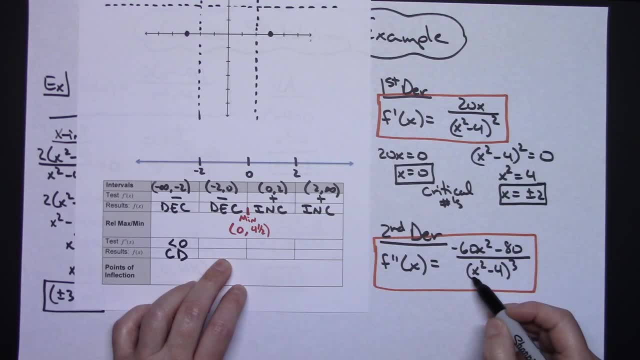 This will be a negative on top. and then plugging in a negative 1 here, Negative cubed gives me another negative. so negative divided by negative, this one's gonna be greater than 0. I almost missed that one. and then that makes the original function concave up. 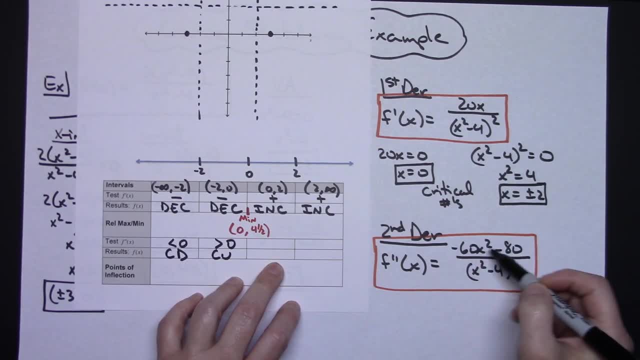 All right. plugging in a positive 1 here will give me a negative on top. Plugging a positive 1 here- negative cubes- still going to be negative. so again, greater than 0 and a concave up on the original function. Now a really large number, so really large number will give me a negative on top. 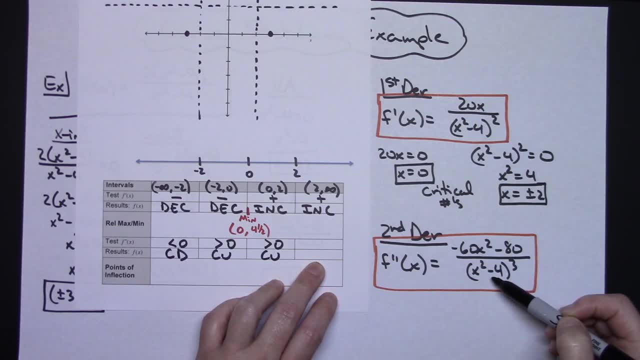 Really large number here is going to give me positive in here. so now I'm back to a less than 0 Negative, which would be a concave down. okay, now, taking a look at this, all right now, from concave down to concave up- That when that change occurs, then we usually have a point of inflection. all right, but this is at negative 2. 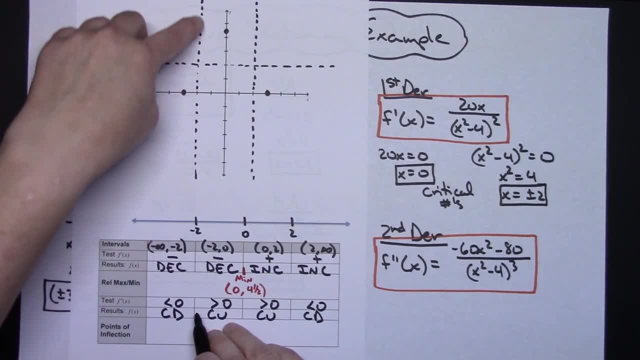 All right, well, at negative 2.. I don't have a point of inflection. I've got a vertical asymptote, So I did not have any there. and then when I switch from concave up to concave down here, This is at 2. 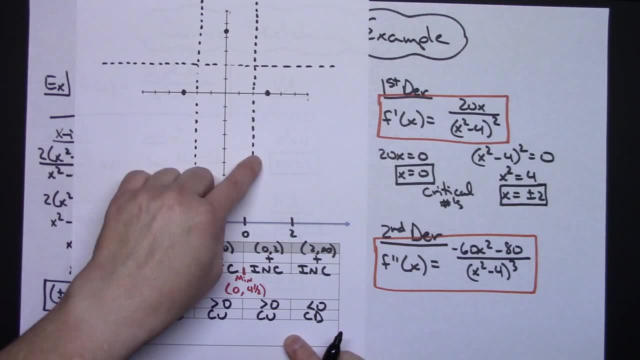 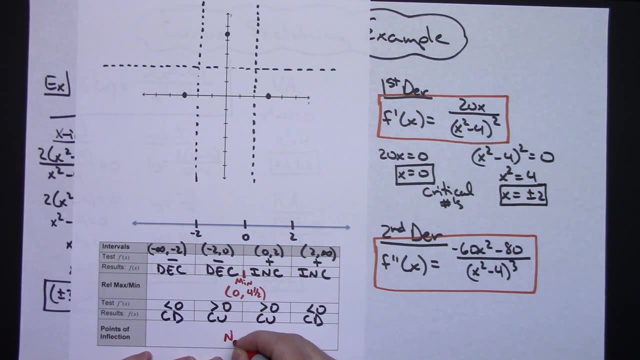 But I already know what's going on at 2.. I have a vertical asymptote at 2. all right, So I do not have a point of inflection. so There are no points of inflection on this one, so we can just put none right there. 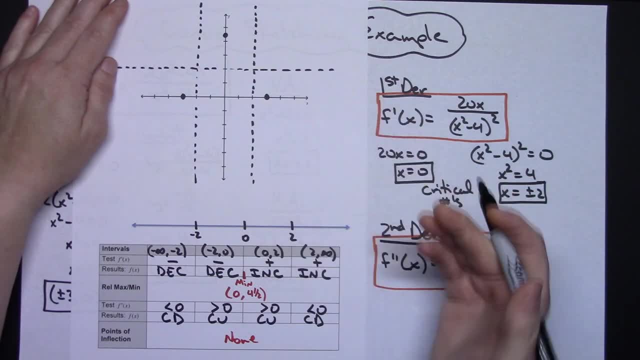 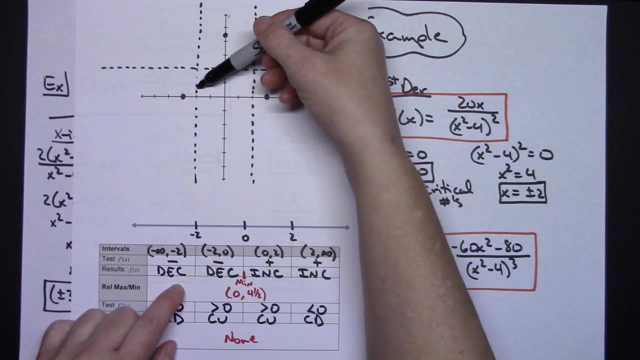 All right, but now you're gonna take the chart and you're gonna finish your sketch. all right. this lays everything out really nice And neat for you, all right from negative infinity all the way up to this negative 2.. I've got to be decreasing. 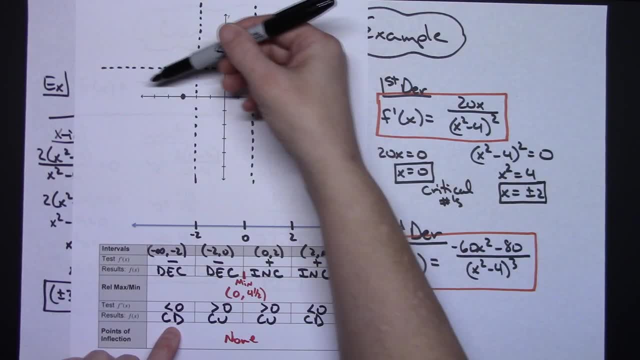 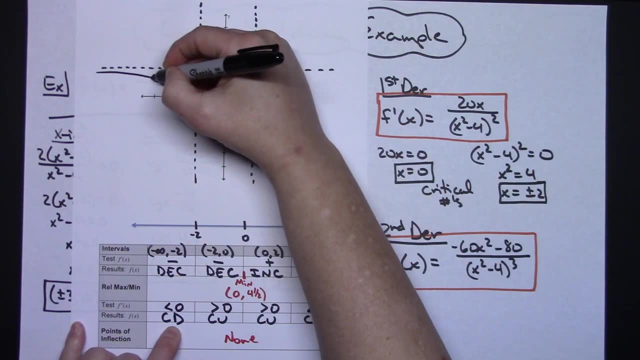 I know I have to go through this point And I need concave up and down, Concave down, all right. well, so if that's an horizontal asymptote, then I got to be coming in this direction, Hugging that asymptote and coming through that point. all right, I am, concave down. 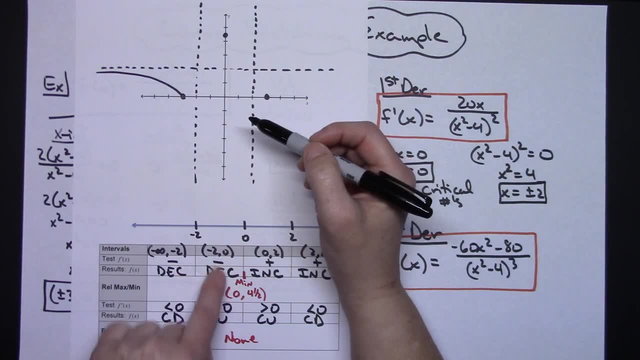 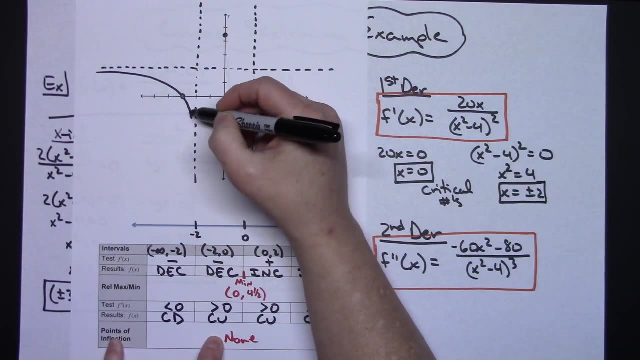 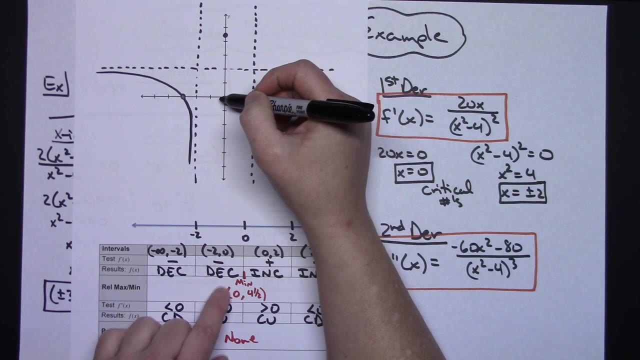 Okay, and I am, the function is decreasing. all right now. taking a look at this interval from the: well, I could even go all the way here. Let's go all the way up to that negative 2 there. Well, yeah, let's go all the way up. better hug against that. all right now. from negative 2 to 0, I got to be decreasing and 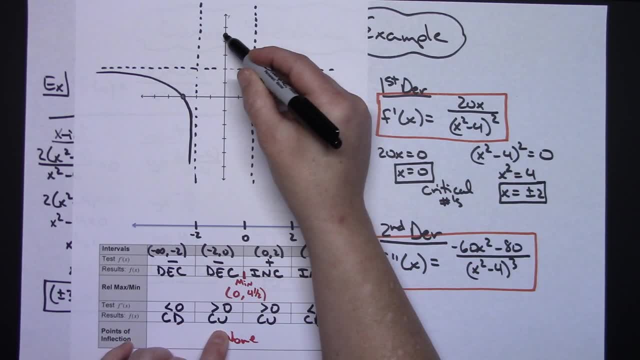 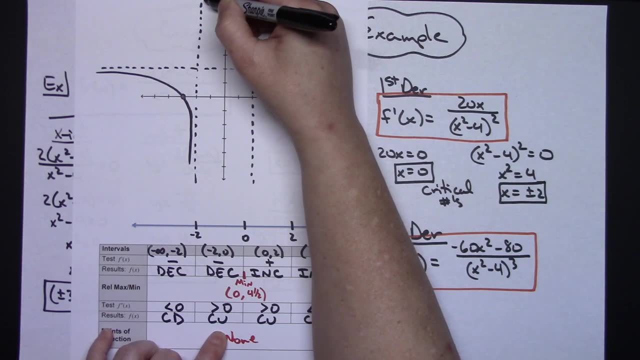 I got to be concave up and this point here has to be a minimum. So to get this being a minimum Decreasing function and concave up- I'm going to have to start all the way up here and hug this asymptote And come down so that that ends up being a minimum, right there. 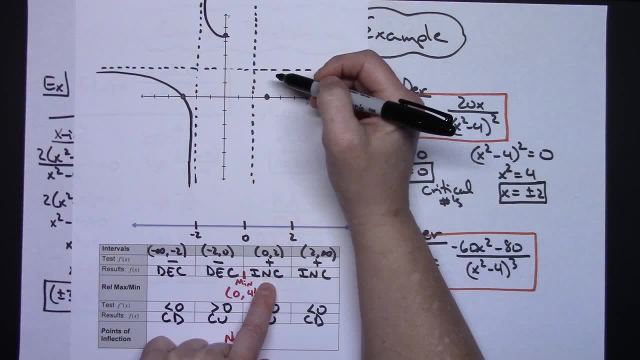 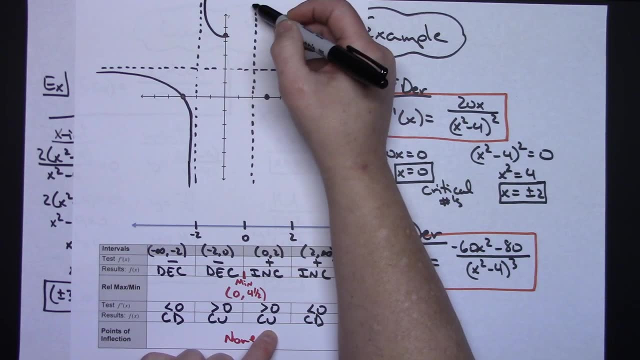 All right, from 0 to 2. all right, I've got to have an increasing function with concave up. this still has to be a minimum here at 0, 4 and a half- All right. so I've got to get increasing and it's got to be concave up. 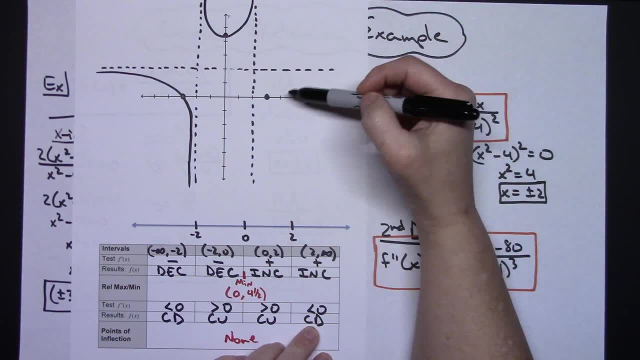 So I'm going to finish that right there. and then, on this last interval from 2 to infinity, I've got to be increasing again, and So increasing can't be down here. increasing it's going to have to be down. here. I got to be concave down. 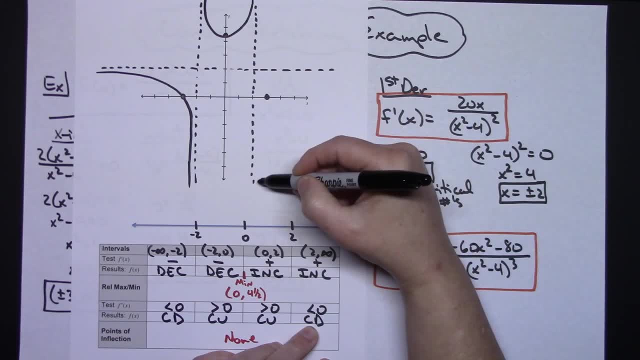 I got to go through that x-intercept right there. I've got a hug here. All right. now let's check and see. yes, I am increasing. it is concave down. I go through that point, okay. So it's a matter of going through each of those. 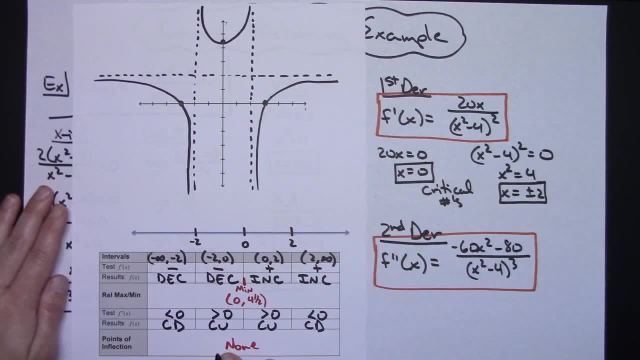 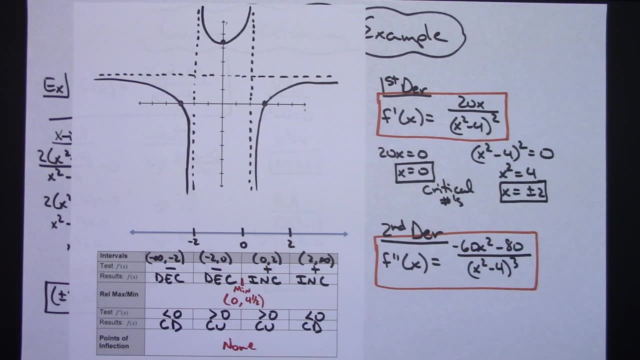 Little intervals and then checking to see what you've got going on there. so I definitely have a minimum. everything is increasing, decreasing, concave up and concave down, like it's supposed to be. so I'm just, you know, a nice example of walking through all the different parts of 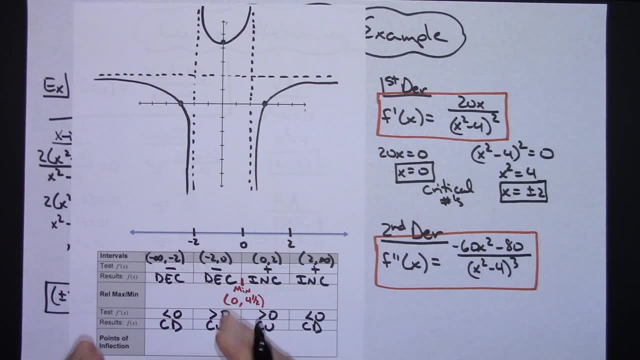 A curve sketching, that you can do Things, lots of things that you can do without any calculus whatsoever and- and it's not till the very end- when you calculate that first and second derivative and you look at the critical points and you Look at the possible points of inflection before you end. 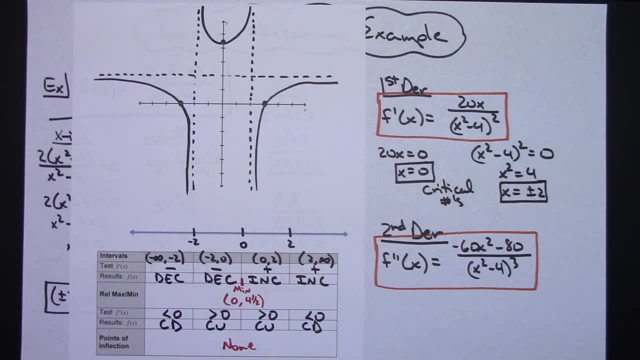 Actually imply some of your calculus there. so definitely thanks for watching and be sure and subscribe to the channel. Thanks,